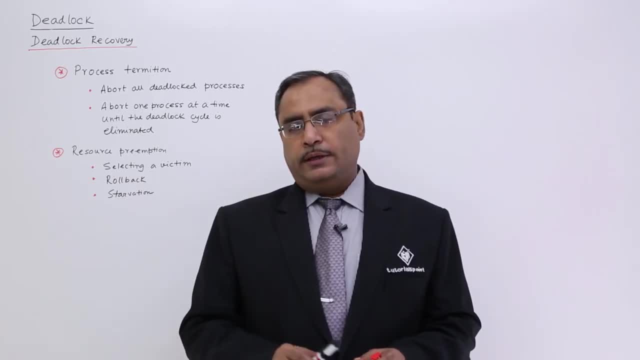 In this session the topic is deadlock recovery. In the earlier video we have shown you, or we have discussed with you that how to detect whether deadlock has occurred in a system or not, And if it has been detected that a deadlock has really occurred, then to retrieve. 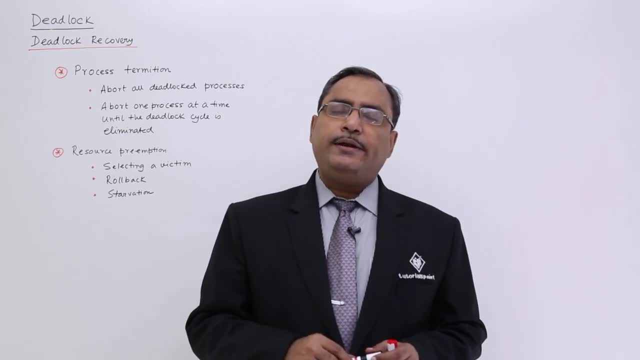 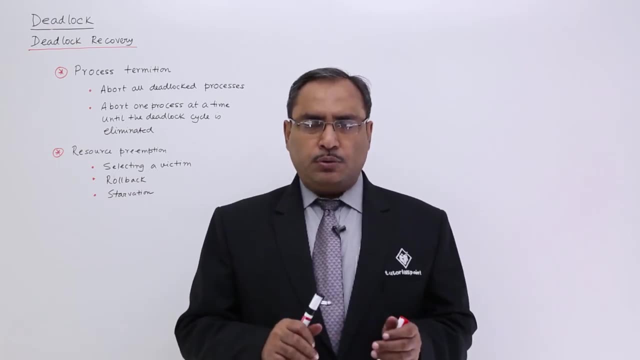 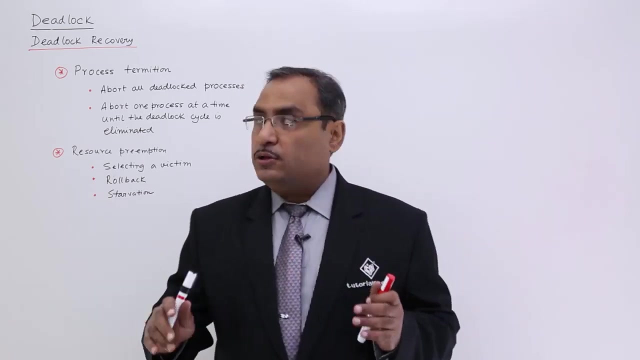 the system from the deadlock situation, we should execute deadlock recovery. The system itself cannot get recovered from the deadlock state. So to get back my system deadlock-free, we are having both mainly two different methods. One is the process termination and other one is the resource. 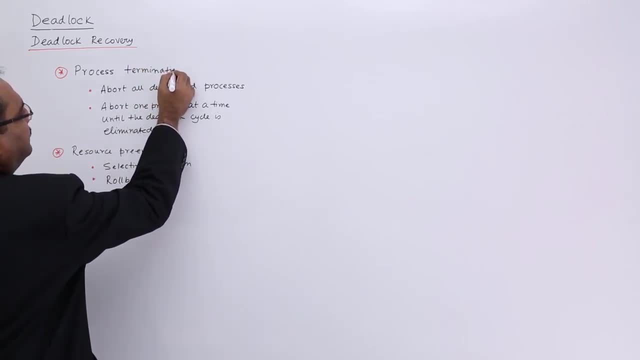 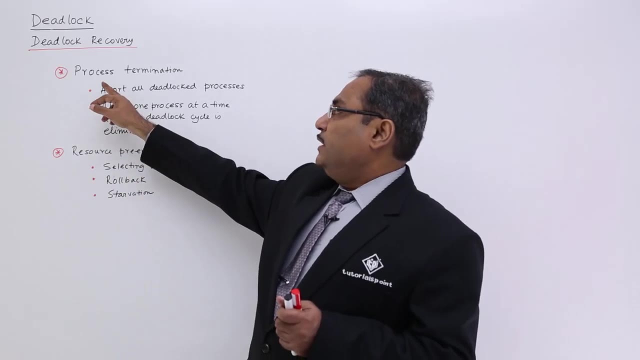 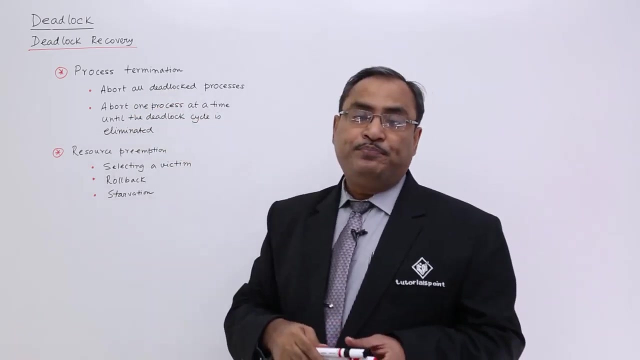 preemption. So let me write this one. Ok, one is the process termination and next one is the resource preemption. So let me go for the process termination at first. process termination: we are having two methods. one is about all deadlocked processes, so process. 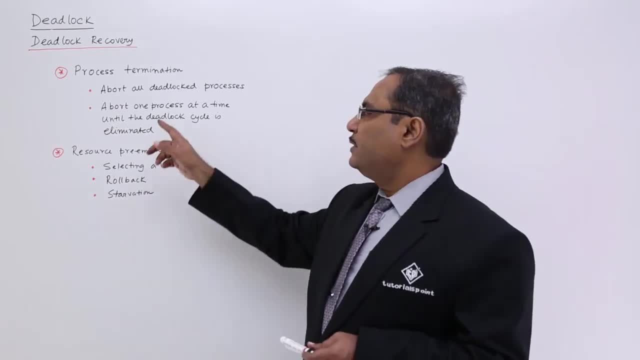 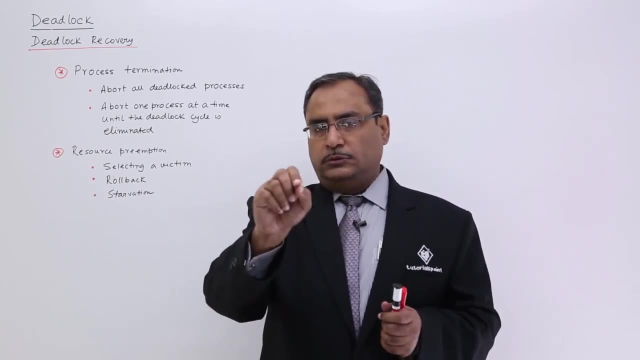 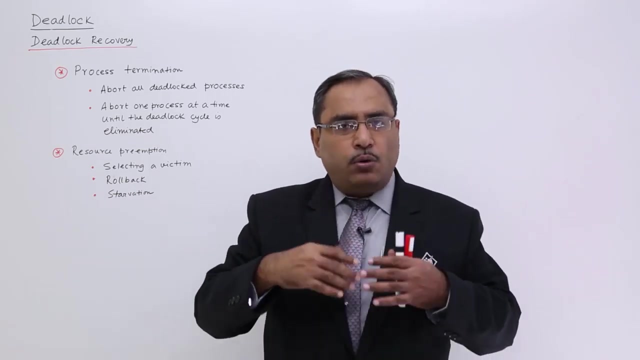 termination means you are killing processes. process termination means you are killing processes. so about all deadlocked processes. that means you are not selecting that i should terminate this one or that one. i shall delete all the processes who are in the deadlock state. so then i shall go for allocation of the resource again. so that is process. that. 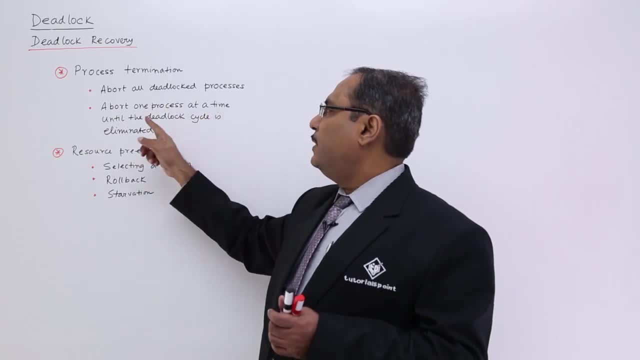 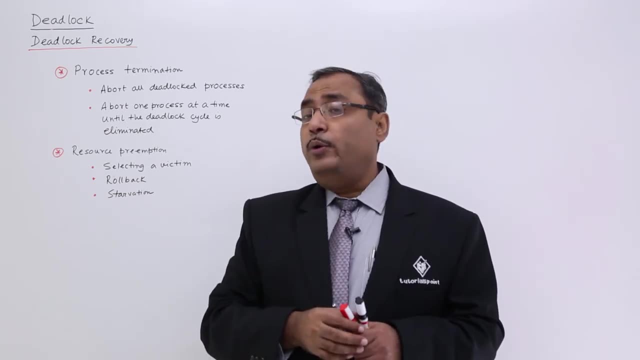 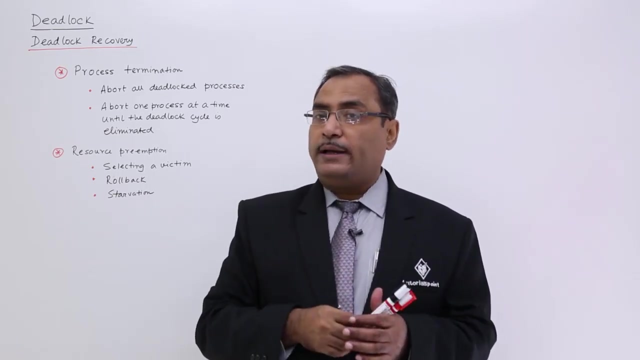 is the one. second one is about one process at a time until the deadlock cycle is eliminated. we discuss the resource allocation graph. we discussed wait for graph. we know that, in case of wait for graph, if there is a closed cycle with a not, the deadlock is bound to take place. 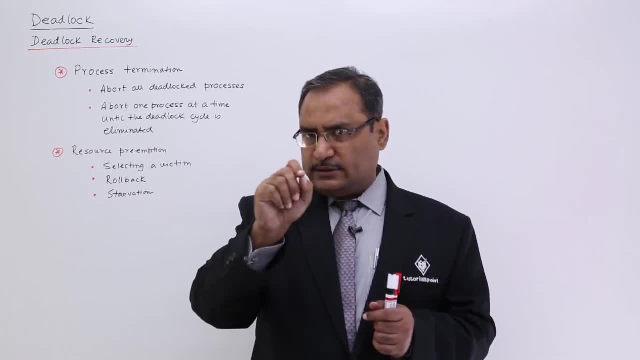 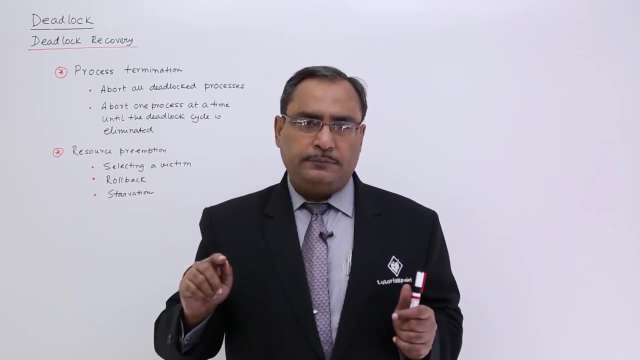 so in that case i shall have to select that, which process i should select and i should kill it, i should terminate it so that the cycle will get eliminated. so about all deadlocked processes, that means you are killing processes, that means you are Ahed. the first process we applied, which is target here, is, in case it is, process operation. 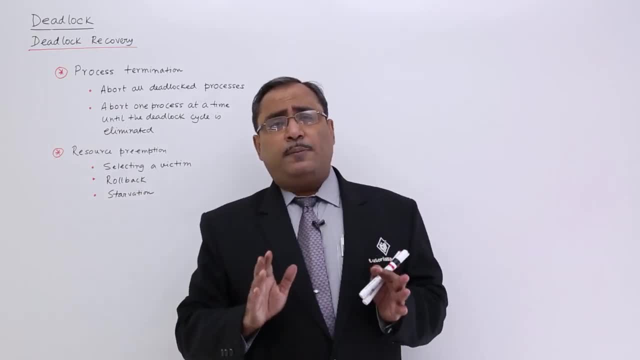 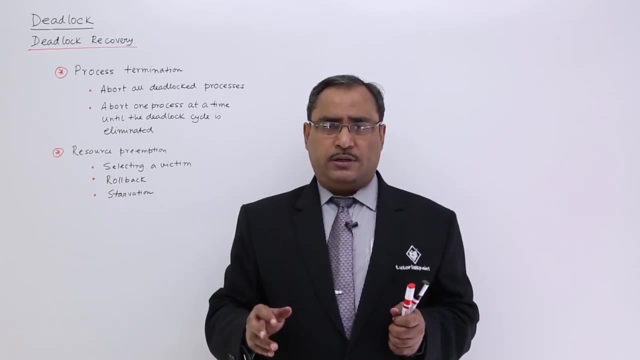 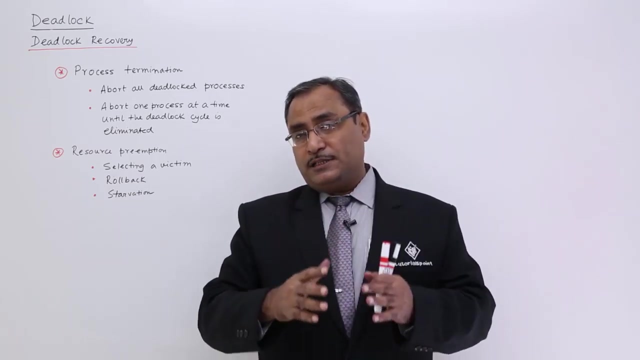 possible. the process Theatre suppose is a particular process which has got execution 90 percent now when it is going to demand or request some additional resources. so now the deadlocked situation has taken place. so 90 percent tasks, 90 percent process completion have been done, has been done, and now you are terminating that one. so that will be a very 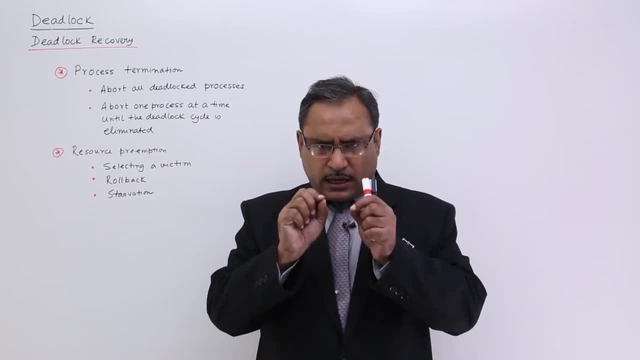 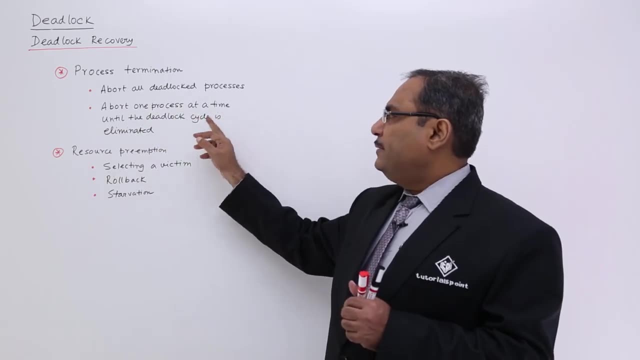 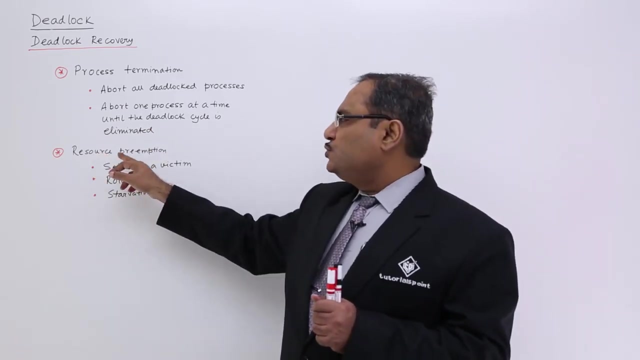 costly affairs for you. so it is better to go for selecting a process if goes away it selecting a certain process, select a certain process which will eliminate the deadlock cycle. so about one process at a time until the deadlock cycle is eliminated. so that is my process. termination category: under the resource preemption, we are having three things. 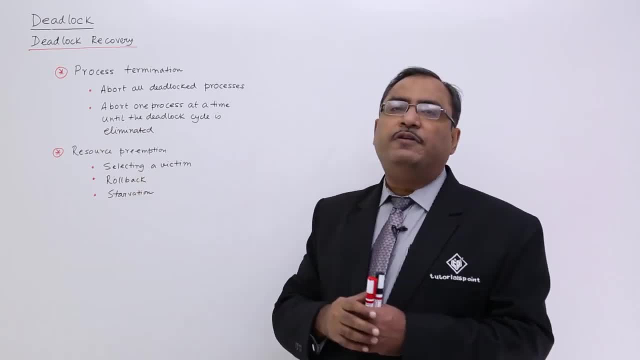 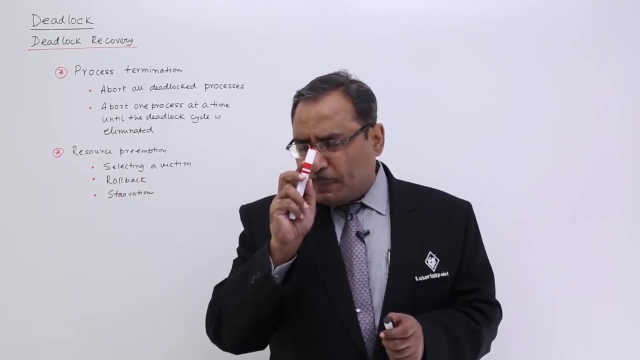 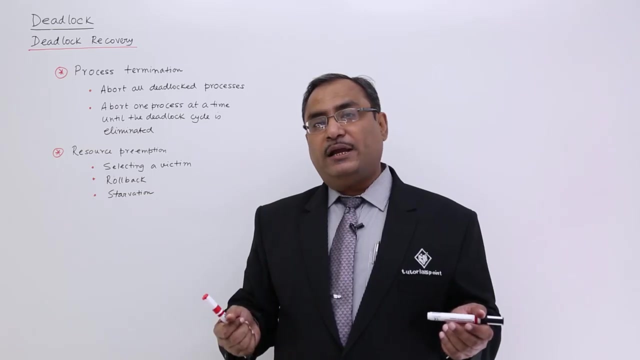 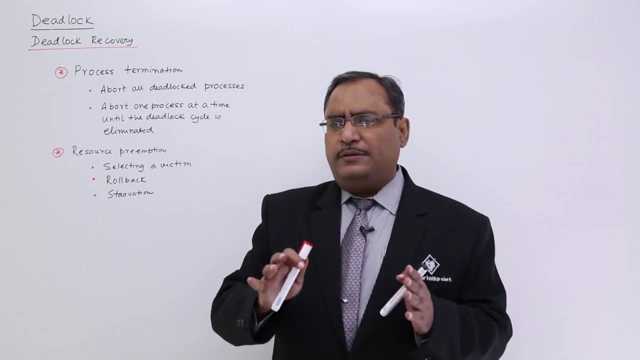 one is the selecting a victim. rollback and starvation. let me discuss one by one. so selecting a victim means in this case, i shall select a particular process from where i shall take away the resources. now, what will happen? if you take away the resources from a process, then it is now again i am. i can say you the same thing. that means when you are selecting. 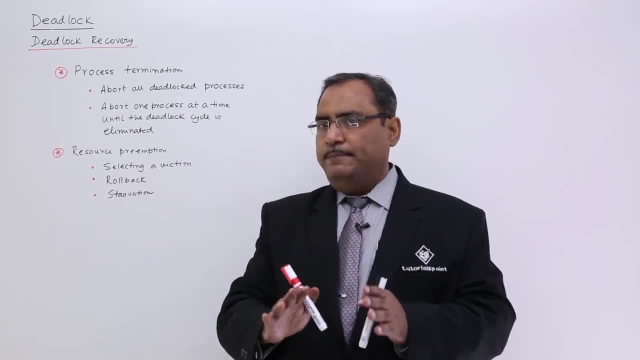 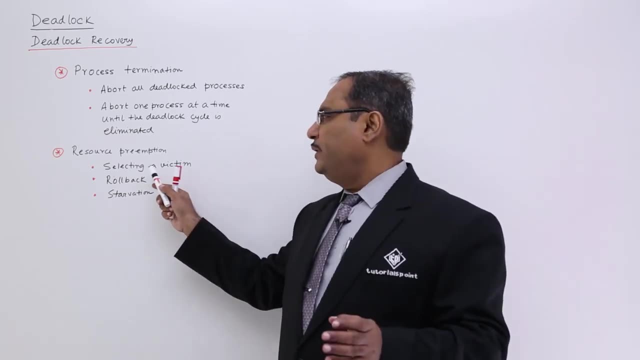 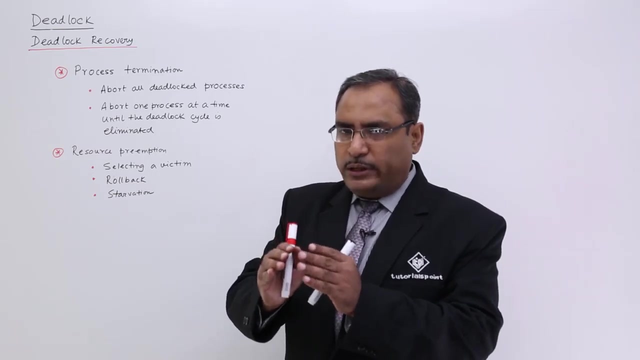 a certain victim, then you should select that very victim, who from whom you are taking away the resources to allocate them to the other waiting, waiting, waiting things. so, selecting a victim, in that case you should select that one, that very process where the cost will be minimum, after selecting the victim and resource preemption. 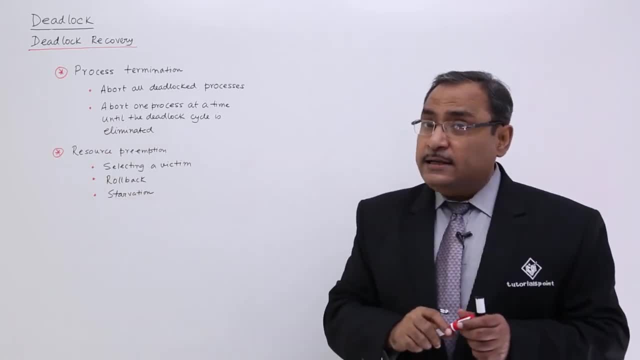 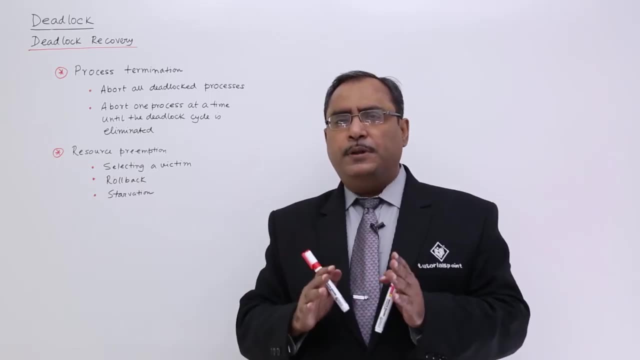 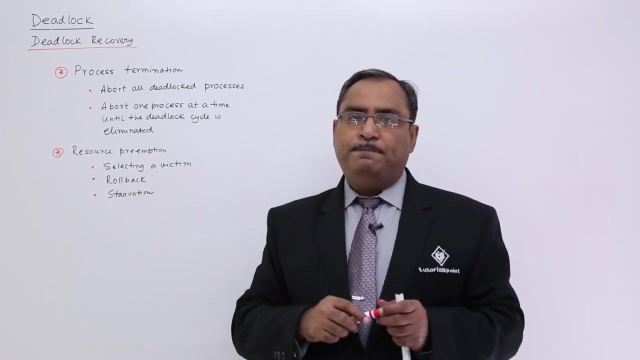 the cost should be always minimum, so that selection must be done very intelligently. as i told you earlier, a process has got almost ninety percent completion. now you are taking away the resources from it, so it will be a costly thing. so that is the same. next one is the rollback. rollback means you did the allocation, you did the allocation. 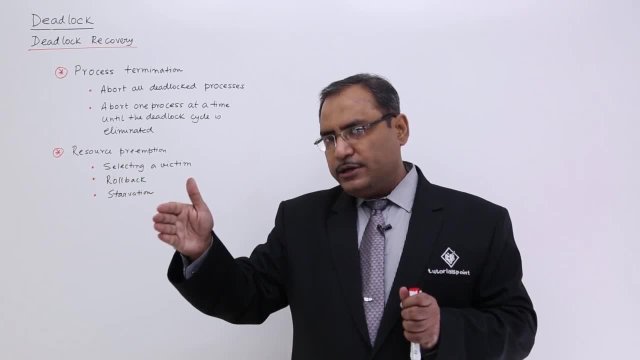 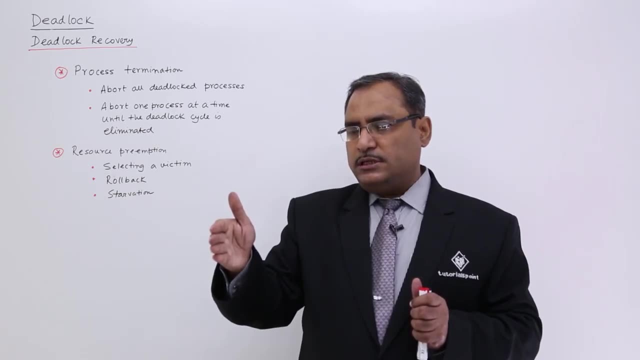 another process has come. you did the allocation. another process has come. you did the allocation. now, the deadlock situation has taken place. now just undo the last allocation to the process. just undo the last allocation to another process. are you in the safe state? yes, now go for allocation. 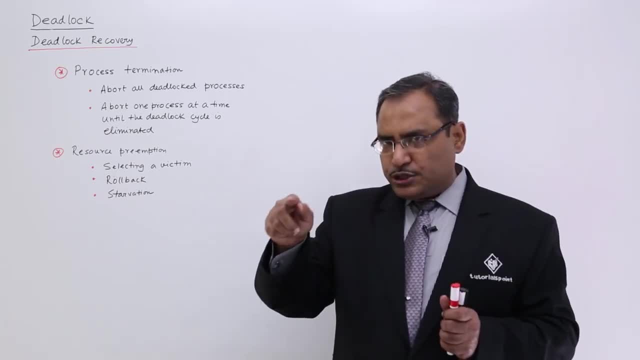 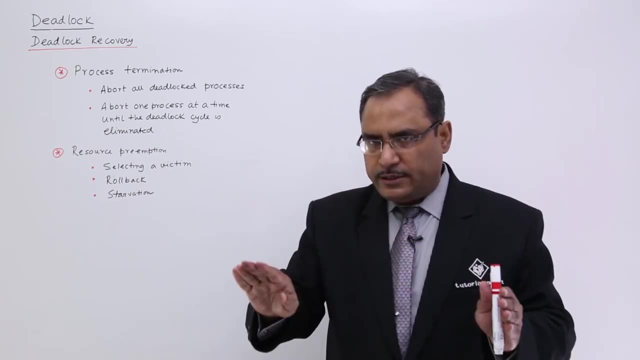 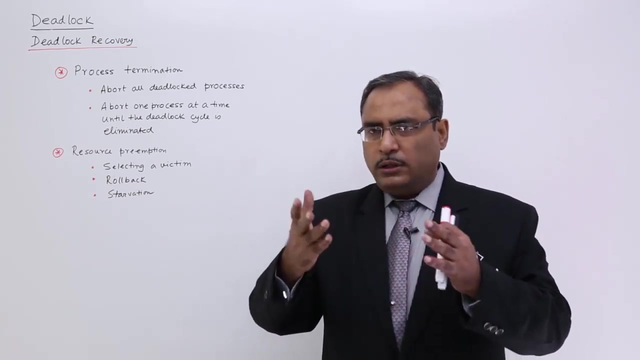 in some different manner. so you did the allocation and now you are doing the rollback. now you are doing the rollback, the system will find that it is now in the safe state. Now there is no need to become worried about the deadlock situations. So now go on the resource allocation to the processes.